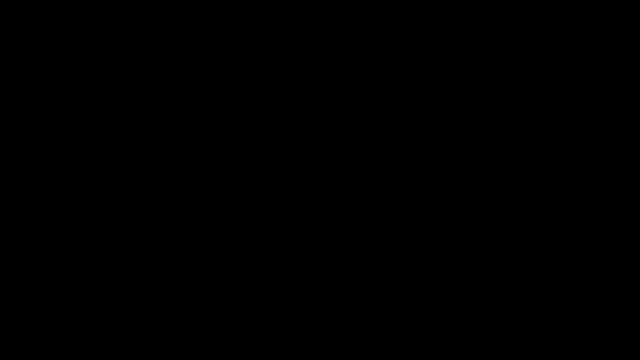 Now this video is a continuation of another video I've created on VSEPR theory: Basic Introduction. you can find it on YouTube. So we're going to focus on the molecular geometry of the trigonal bipyramidal structure. Now this structure has a central atom and it has five other atoms attached to it. 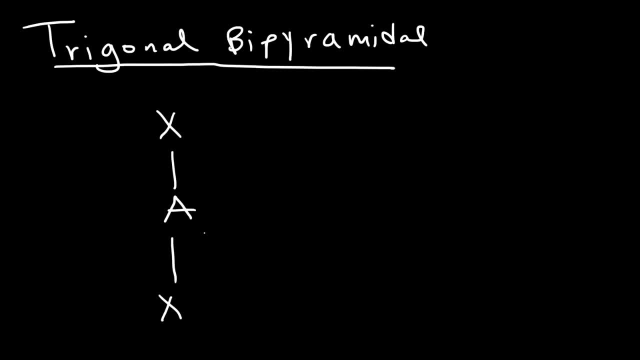 So you have one on top and one on the bottom. Now the bond angle between those two atoms is 180.. Now there's three other atoms that you need to worry about, which looks like this: Now, those three atoms, they have a trigonal planar shape. 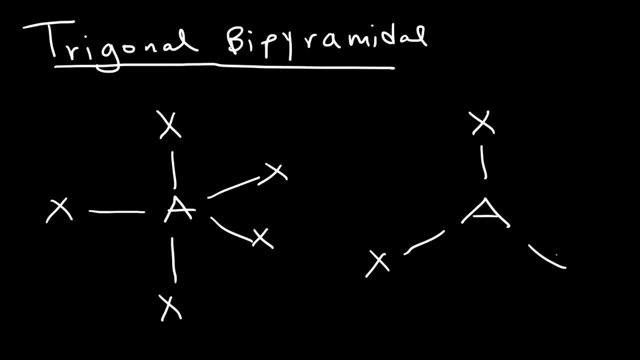 If you focus under on those three atoms, it would look like this: And so the bond angle between these three is 120.. And the bond angle between these two is 90. So there's three angles that you need to know for the trigonal bipyramidal shape. 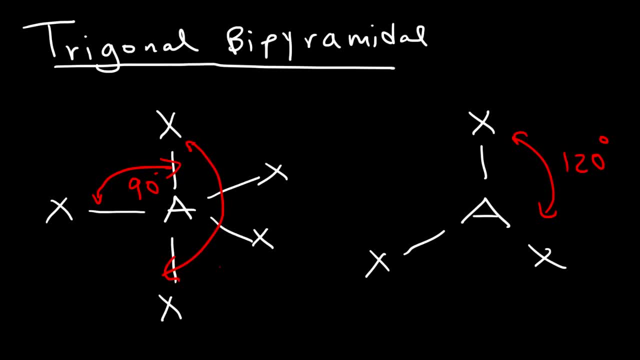 That angle is 90,, between these two is 180, and the three in the middle, that's going to be 120.. A good example of the trigonal bipyramidal structure is PCL5, phosphorus pentachloride. So if you look at the trigonal bipyramidal structure, you'll see that it's a trigonal bipyramidal structure. So if you look at the trigonal bipyramidal structure, you'll see that it's a trigonal bipyramidal structure. 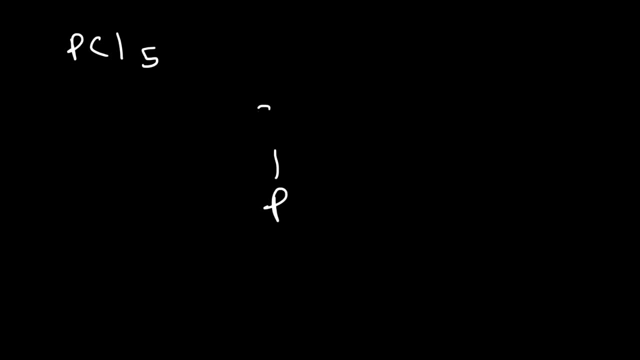 So in this structure phosphorus is at the center, We have two chlorine atoms in- let's call this the Z direction, And then we have three chlorine atoms in the XY plane. Each chlorine atom contains three lone pairs, So the total number of valence electrons in this structure is actually 40.. 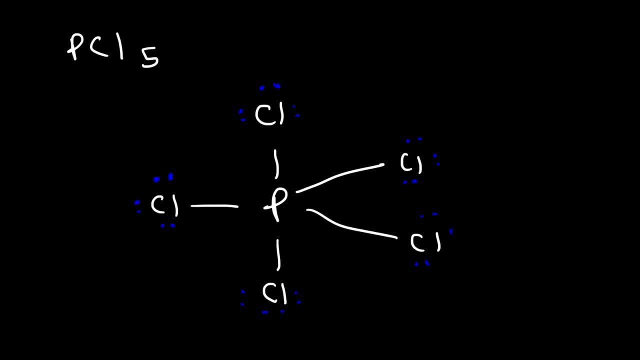 And so that's the trigonal bipyramidal structure. And so that's the trigonal bipyramidal structure. And so that's the trigonal bipyramidal structure. So that's one example of a trigonal bipyramidal structure. 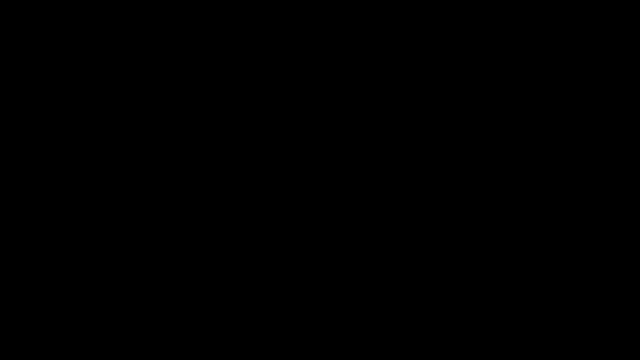 Now there's some other structures that you need to be familiar with. The next one is the seesaw. Now you can get a list of all the molecular geometries and their shapes that you need to know if you go to Google Images and type in molecular geometry. 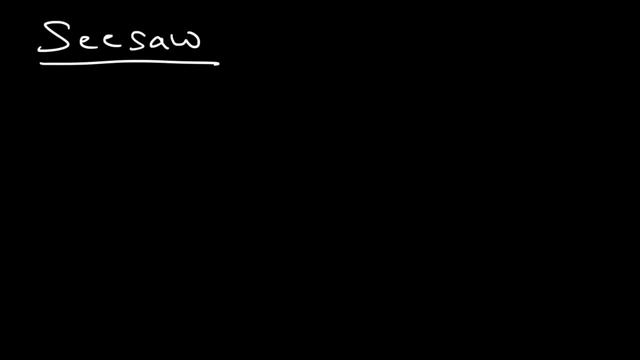 I believe it's the first one in the upper left And you should see all of the geometries And it's nicely listed for you. So if you print out that page, I think it's going to help you tremendously. Now in the seesaw structure you have a central atom. 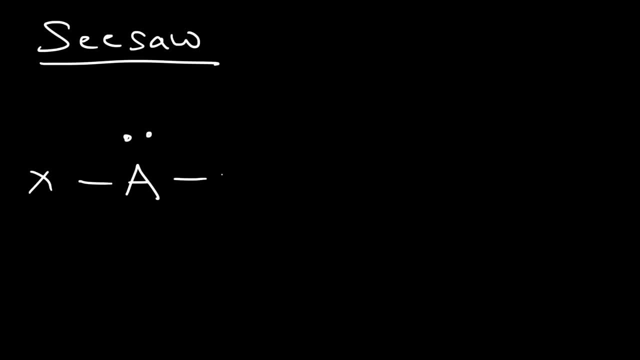 And it has a lone pair with four other atoms. You can draw it like this, Or sometimes you might see it written this way: So that's the seesaw molecular geometry, And one good example of it is sulfur tetraphy. 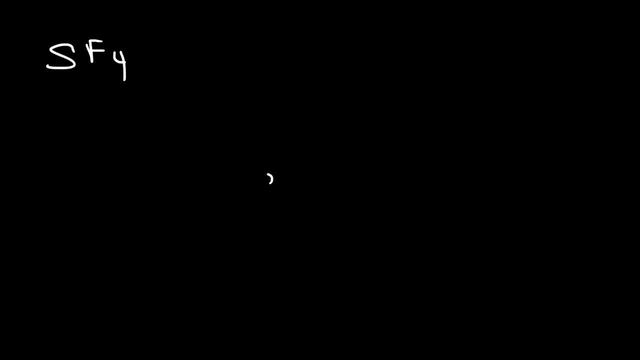 It contains one lone pair of atoms, and it's attached to four fluorine atoms, And each of those fluorine atoms also contains lone pairs, But they contain three instead of one, And so that's one example of the seesaw molecular structure. 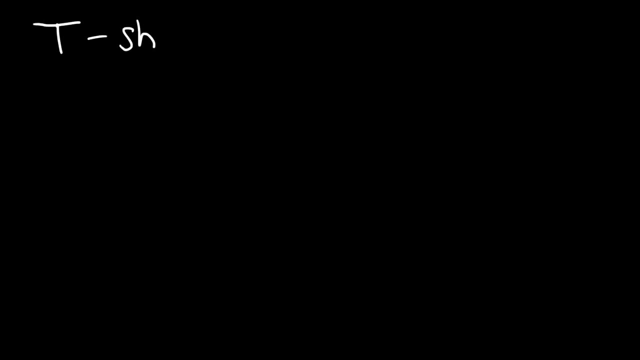 Next up we have the sulfur tetraphy. Next up we have the T-shaped molecular geometry. So what do you think this structure looks like? Well, it actually does have a T-shaped structure. So one way you can draw it is having the center atom placed like that. 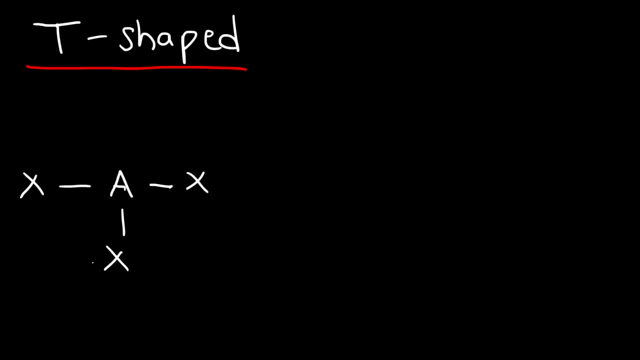 And there's three other atoms attached to it And attached to the center atom there are two lone pairs. So that's the structure of the T-shaped molecule And you can see the T-shaped And you can see the T-shaped in the molecule. 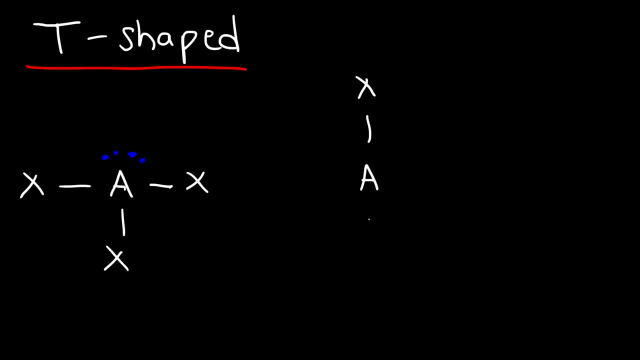 Now, granted, you can also draw it this way too, if you want. So there's different ways in which you can orient the molecule, But this looks more like a T-shape. So what's one example of the T-shaped structure? 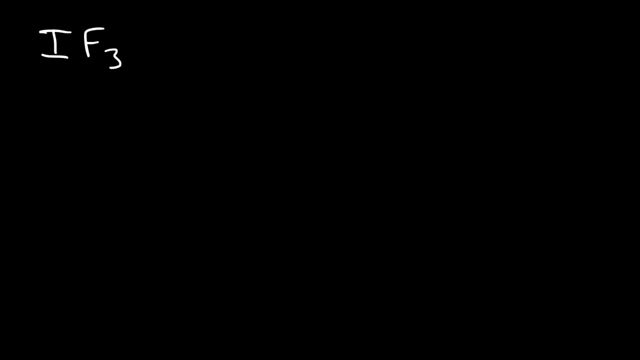 This includes iodine trifluoride, By the way. for those of you who may want to know how to determine the number of Lewis structures in a certain molecule, here's a technique that I use. First I count the valence electrons. 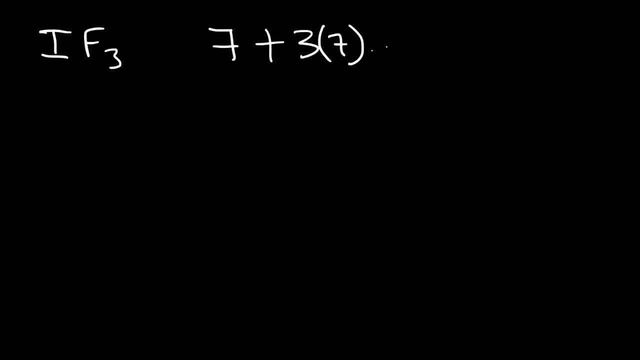 Iodine has 7, and fluorine has 7 as well. Now 7 times 3 is 21, plus 7,, that's 28.. Now fluorine wants to have 8 electrons, So there's 3 fluorine atoms. 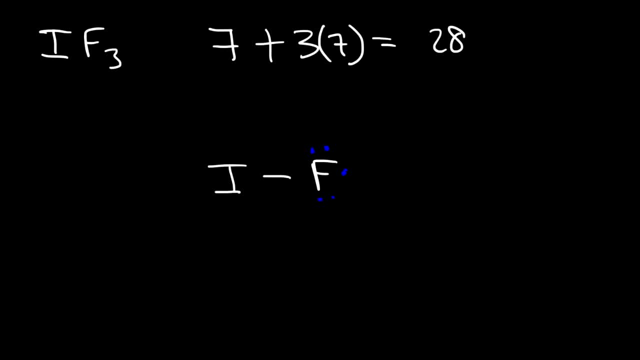 So each fluorine is going to have 8.. So times 3,, that's going to be 24.. So right now I have a total of 16 electrons. Remember, each bond represents 2 electrons. Now in order to get 28,, I need to add 2 lone pairs. 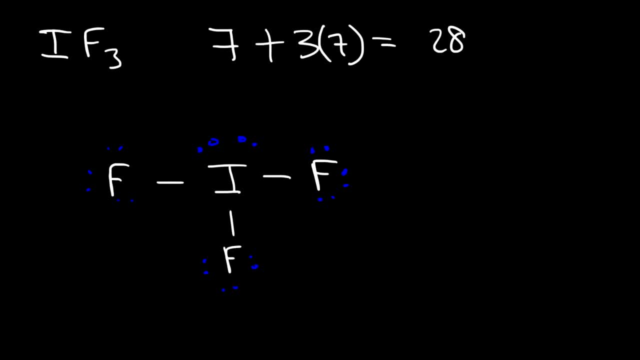 So now it adds up to 28.. That's how I know that there's 2 lone pairs. And as long as this atom is not hydrogen, these atoms will always have 8.. So using the multiple of 8 rule. 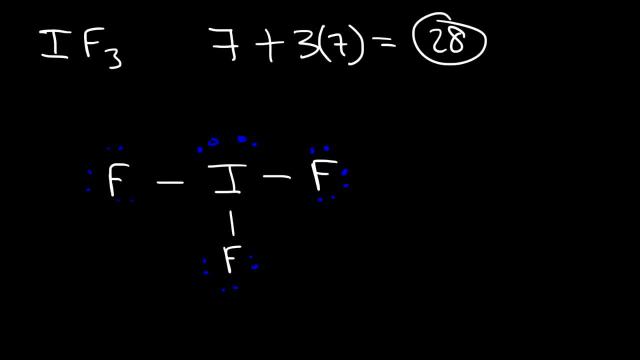 looking at 28,, I try to find the highest multiple of 8 just under 28,, which is going to be 24.. So if you subtract 28 by 24, this gives you the number of electrons that is on the center atom. 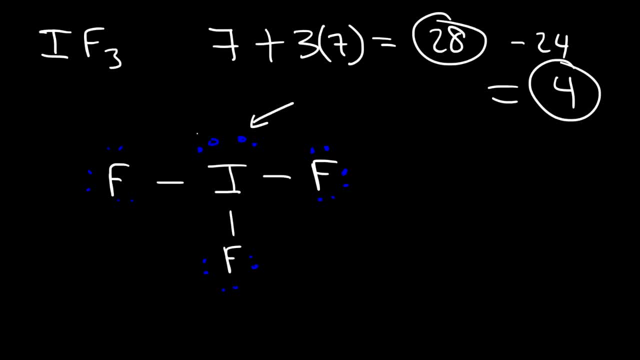 So 4 electrons equate to 2 lone pairs, And that's how you can determine how many lone pairs should be on the center atom. And so this structure is the T-shaped molecular structure. So IF3 is one example of it. 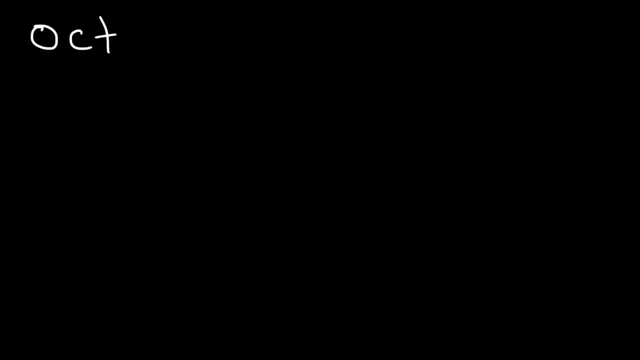 Now the next important structure that you need to know is the octahedral molecular geometry. So you're going to have an atom at the center with 6 other atoms surrounding it. Now the bond angle between these 2 atoms is 90 degrees. 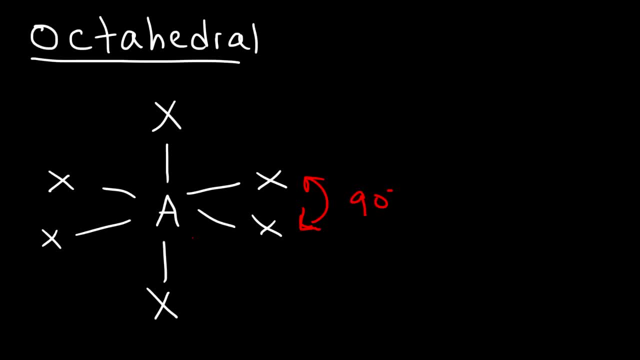 Because 360 divided by 4 is 90.. These are equally spliced In the same plane And the bond angle between these 2 is also 90. So you can view this as being in the Z direction and this as being in the XY plane. 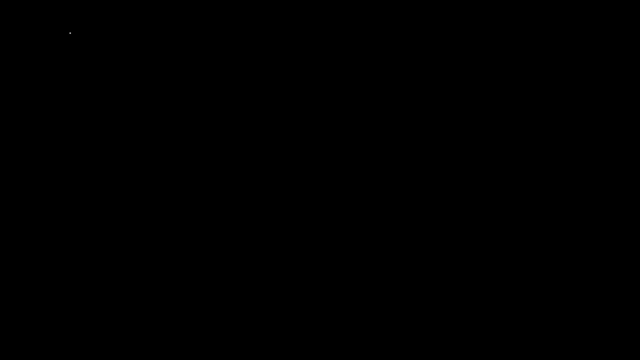 One example of the octahedral molecular structure is sulfur hexafluoride. In this structure, sulfur is attached to 6 fluorine atoms, And so it looks like that And you could easily tell if it's going to be octahedral. 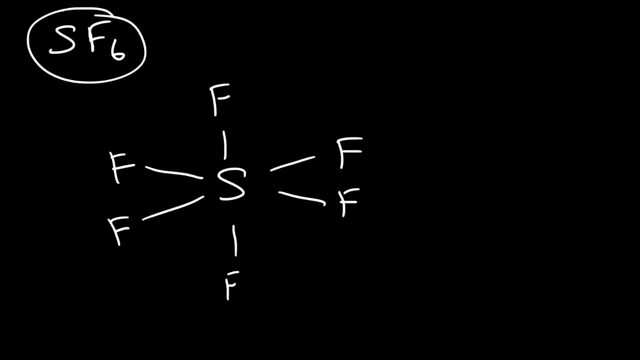 If you see an element with 6 other atoms attached to it and there's no lone pairs on the central element, then it has an octahedral structure. Now, the next one we need to talk about is the square pyramidal structure. 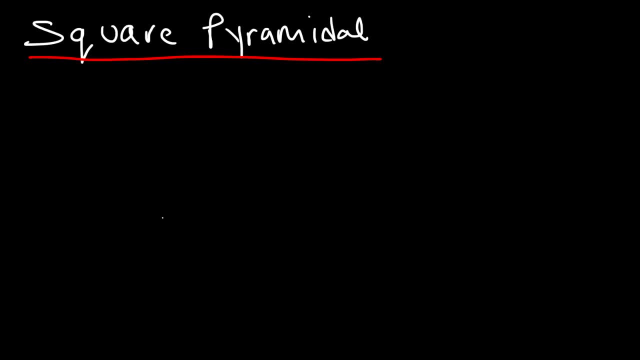 So the general features of this structure is that, attached to the central atom, you have 5 other atoms on it, So it's very similar to the octahedral structure. The only difference is one of the atoms has been replaced with a lone pair. 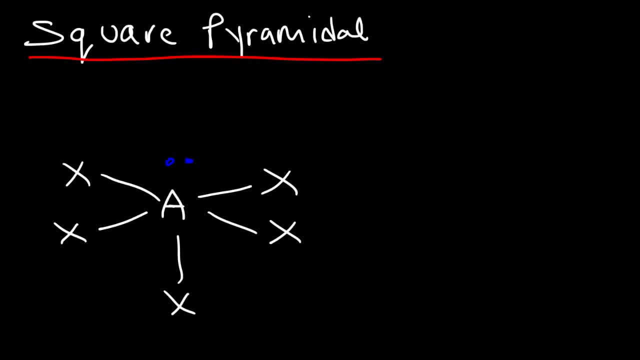 So instead of having 6 atoms attached to the central atom, as in the case of an octahedral structure, you now have 5 atoms attached to the center atom with 1 lone pair. So an example of this molecular geometry includes: 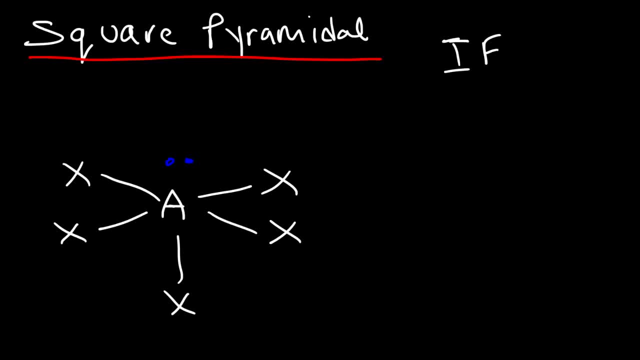 the iodine tetrafluoride- I mean not tetra but pentafluoride molecule. So in it you have iodine at the center with 5 fluorine atoms attached to it And on the iodide item you have 1 lone pair on it. 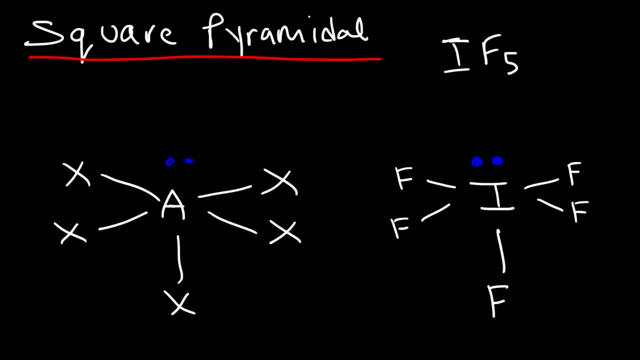 And so it has a square pyramidal molecular structure, And so it has a square pyramidal molecular geometry. Now, the next one, nonetheless, is the square planar structure. Now, it's going to have 6 things attached to it. 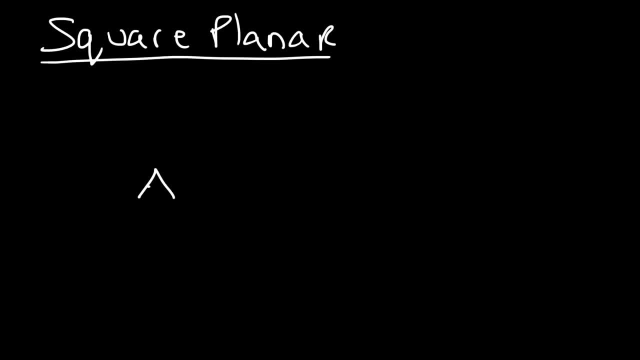 like the octahedral structure, but 2 of those atoms is replaced with lone pairs. So you're going to have 4 atoms attached to it with 2 lone pairs. So there's going to be 1 lone pair on the top. 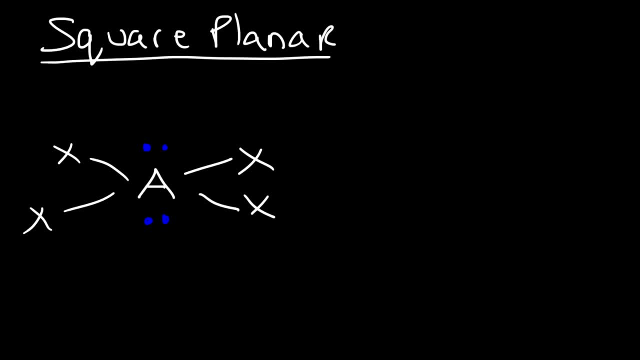 and 1 on the bottom. So that's the square planar molecular structure And xenon tetrafluoride has that structure. So xenon is going to be at the center and it's attached to 4 fluorine atoms. 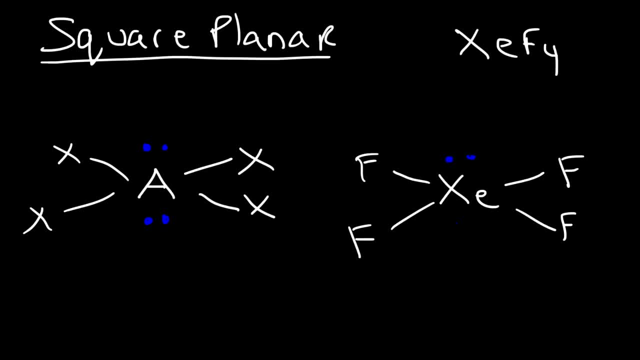 And xenon is going to have 2 lone pairs, 1 above and 1 below. So that's the square planar molecular geometry. So now you know that you have 2 atoms attached to it and you know the most important structures.